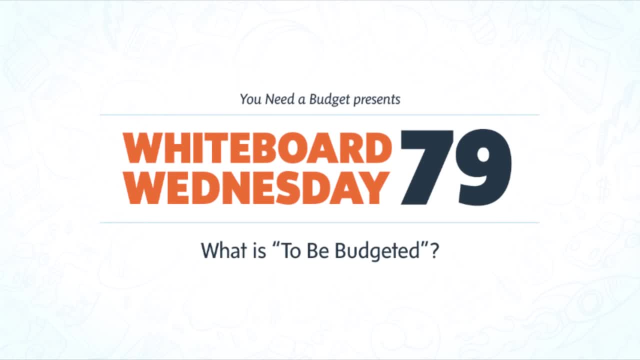 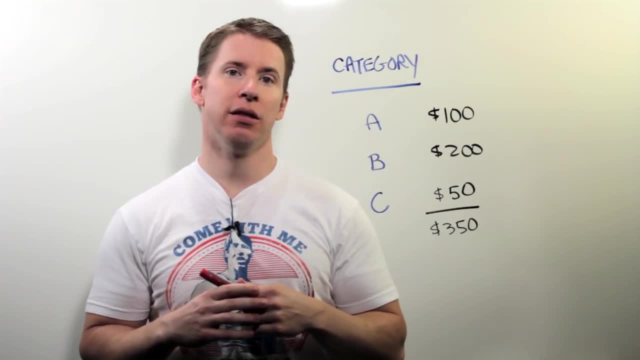 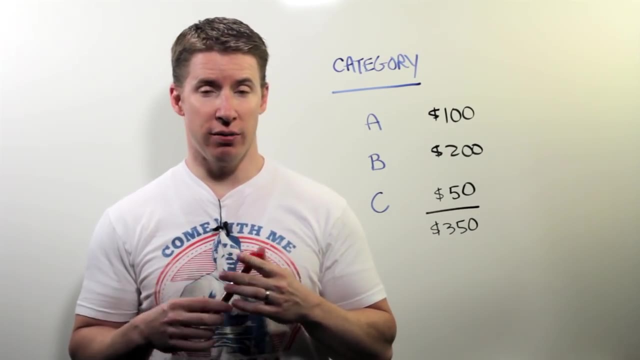 Hello YNABers. My name is Jesse Mecham from YNAB. It stands for: You Need a Budget, You do, And we try and keep the budget fairly simple. Oh, by the way, this is another Whiteboard, Wednesday. 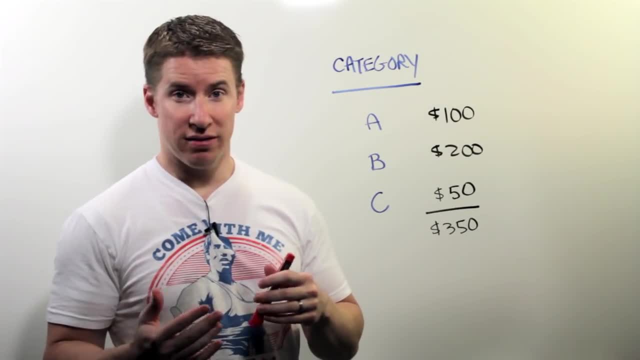 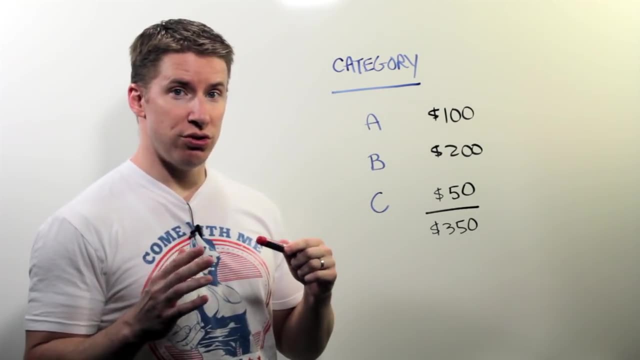 I'm glad to be back. We try and keep it simple. We try and keep the math simple. It is just pluses and minuses for the most part, occasionally an average thrown in here and there. But I want to talk, and I've talked about this before, but I want to talk about it again and just kind of give. 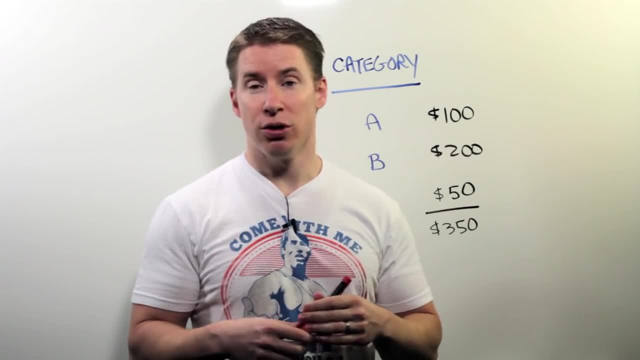 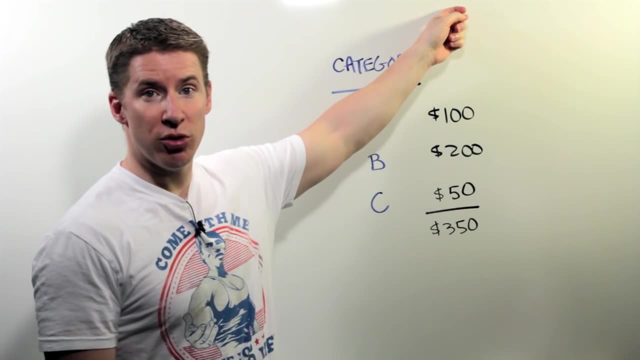 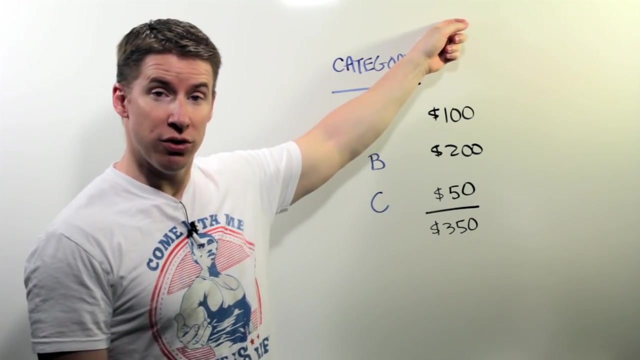 you a glimpse into what we're thinking about currently. This spawned from my desire to change the calculation of that to-be-budgeted number. that's the top of your month And it's green if it's positive and if it's red if you've over-budgeted, And it's a little bit confusing. It's a tough. 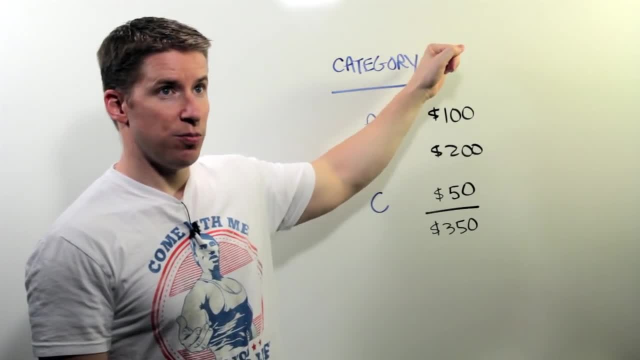 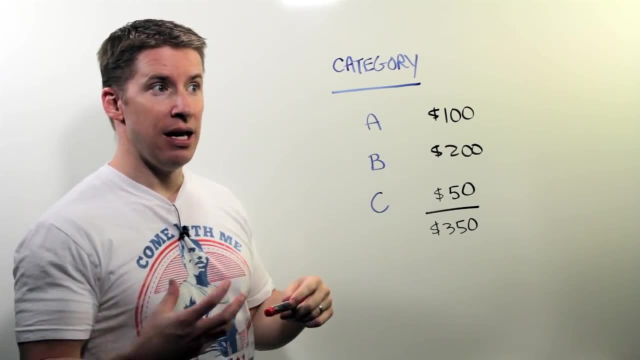 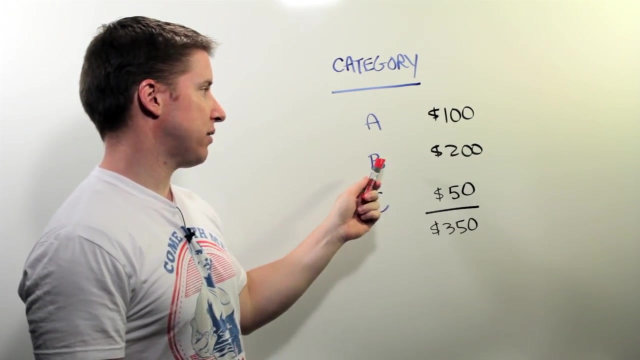 number to get your head around. So this has kind of come from that, with some experiments that have failed, frankly. And now I'm back to the drawing board. I want to talk about a core principle of the software and just a little bit of math. So if you have category A with $100, B with $200, and C with 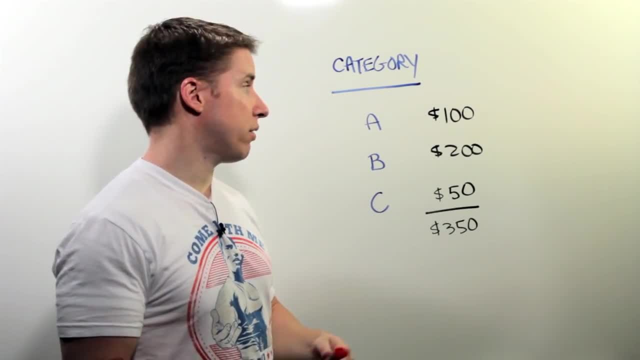 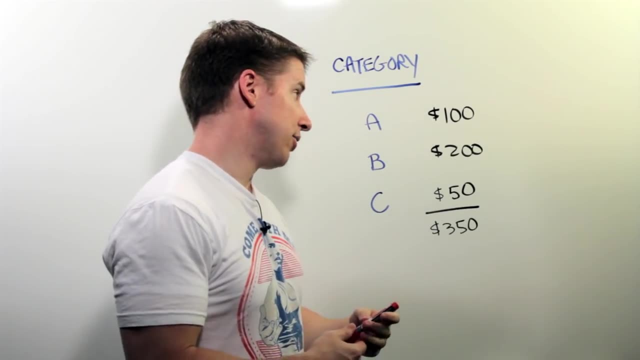 $50, you have total cash on hand of $350.. If you spend $100 in A, you're good. If you spend $200 in B, you're fine, And you can still spend $50 in C. Now, if you decide to spend $100 in C, 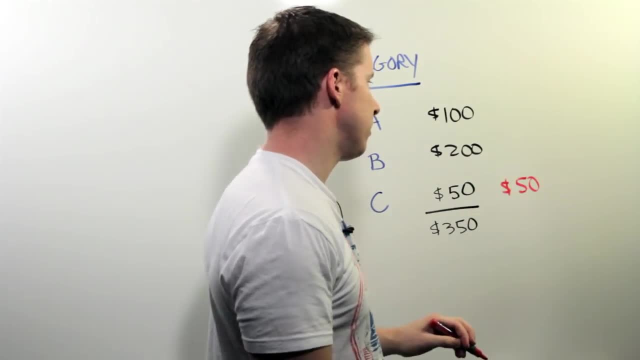 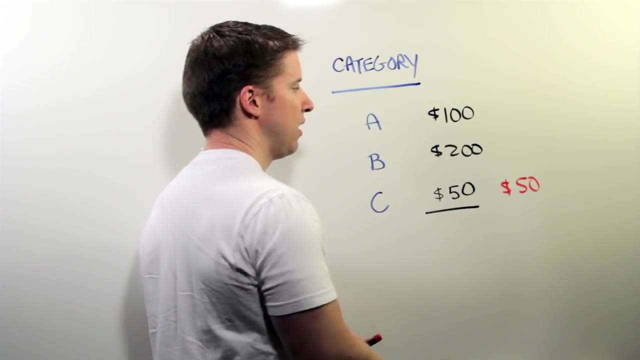 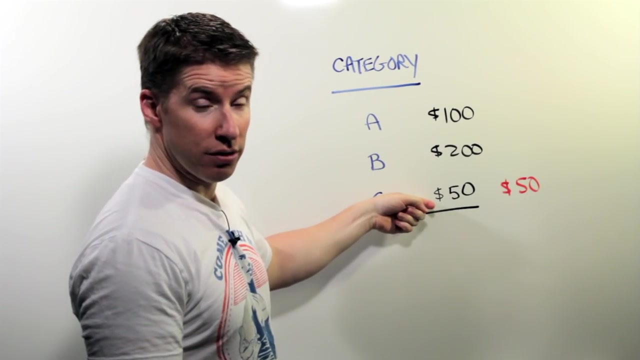 we're going to basically put you in the red $50 there. What do you have as far as cash on hand? Let me erase this with my thumb: Instead of $100, $200, so the $350 here. you've spent $100. So you're. 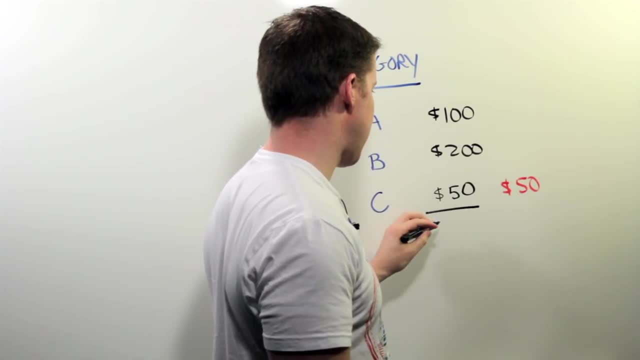 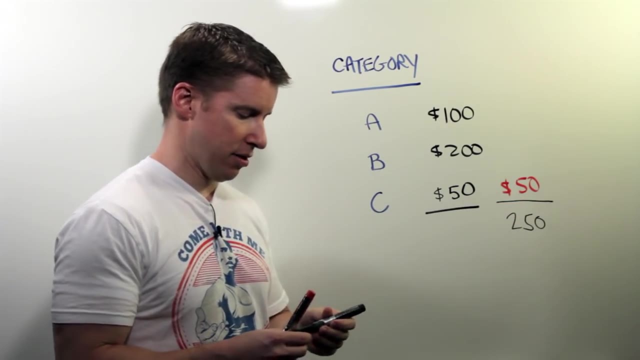 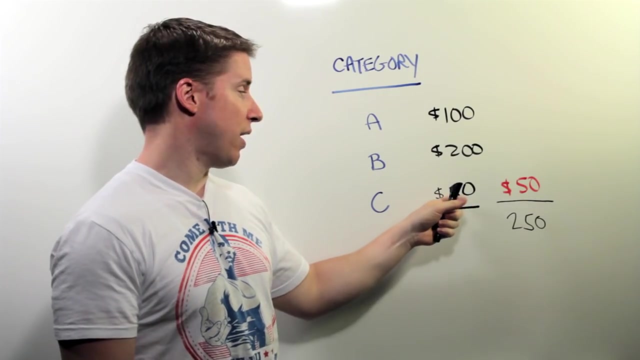 down to $250, right? So actual, real cash on hand- and I'll put it over here- is $250.. This is where my handwriting gets bad, because I didn't Have it all perfect and prepped With $250 cash on hand because you spent $100. Remember you had a? 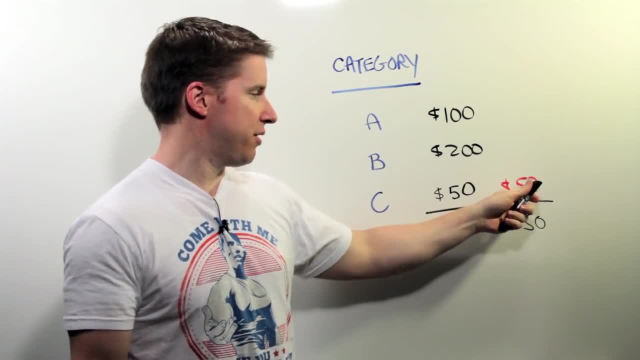 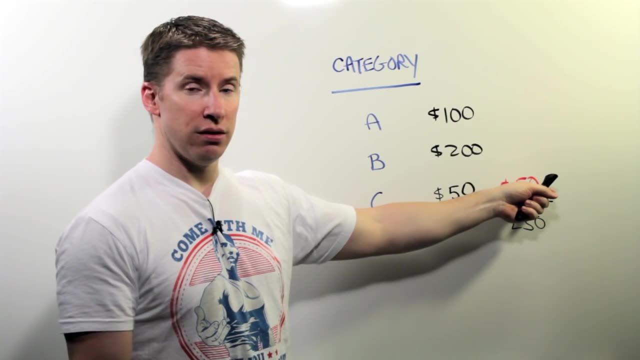 positive $50, and you dropped it down to a negative $50.. Everyone's done this right. You see this in your budget all the time, So you're negative $50 there. So $100 plus $200 is $300, minus $50 is $250. 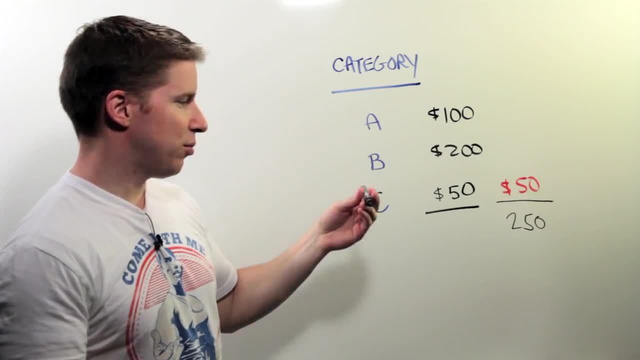 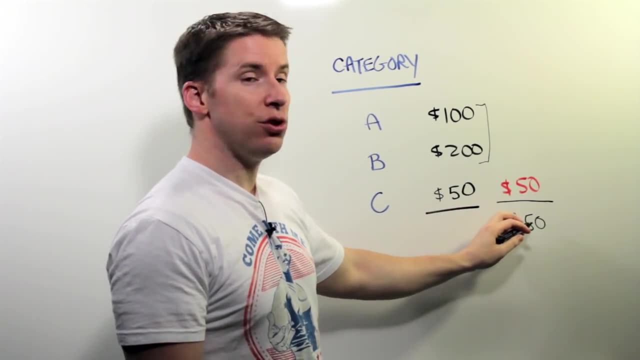 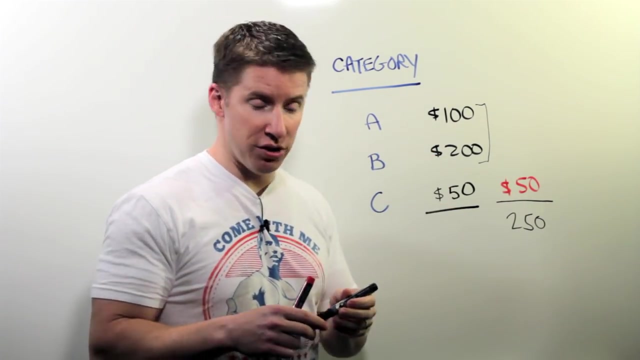 $300 minus $50, $250.. But this is the problem, and this is probably maybe a review for some and first time for others. We're saying you do have actual cash on hand of $250. But we're saying here that A has $100 that you can spend and B has $200 that you can spend. So if you were to just 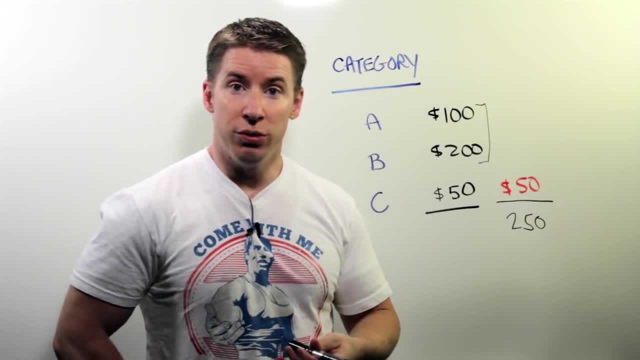 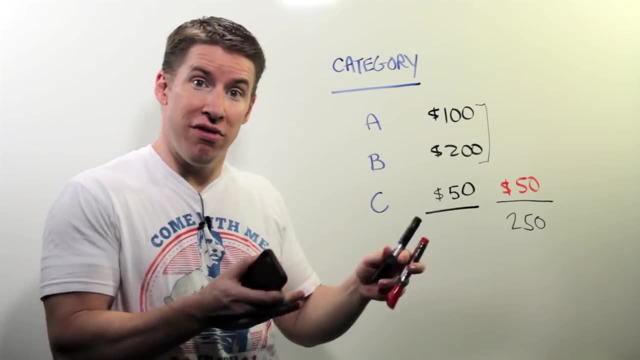 follow your budget and we always say: check your category balances. We say: pull out your phone and look at the category balance and see what it is, and then you can spend that much. So if you were to follow that part of the 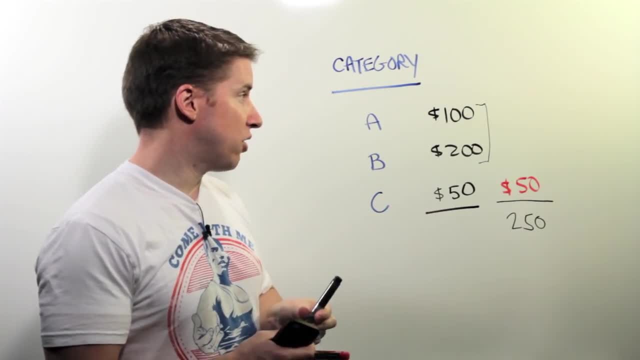 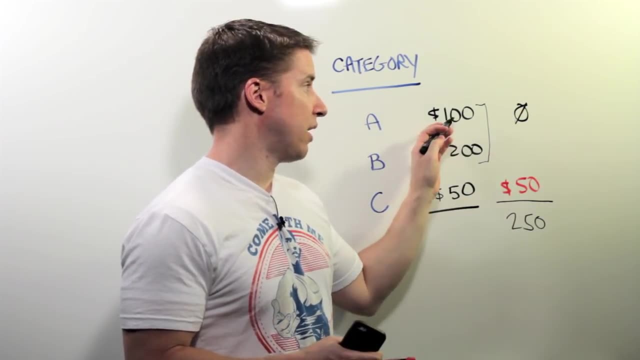 advice. you'd say: oh, I have $100 in A so I can spend that, So you spend all of A, you get that down to $0, and then now you don't have $250 left. you have $150 left because you spent $100. 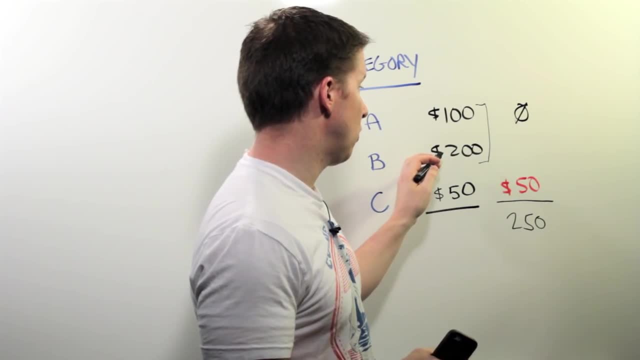 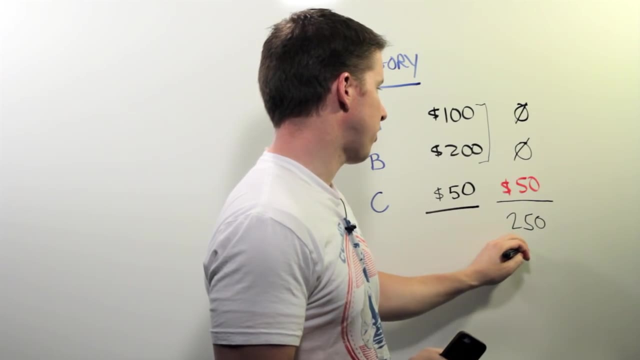 And then you spend another $200 there. so minus $200 there That goes down to $0.. You're at minus $50 overall. We just spent $300.. So if I subtract the $300, we're overdrafted by $50.. 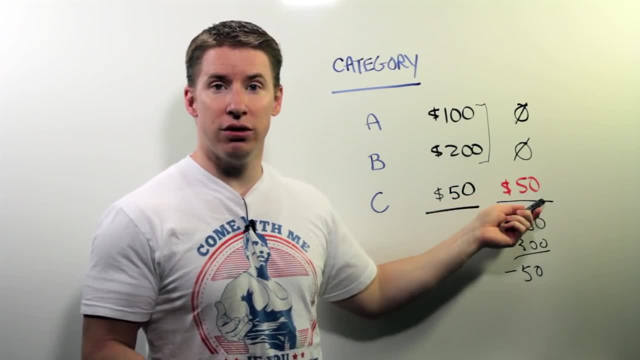 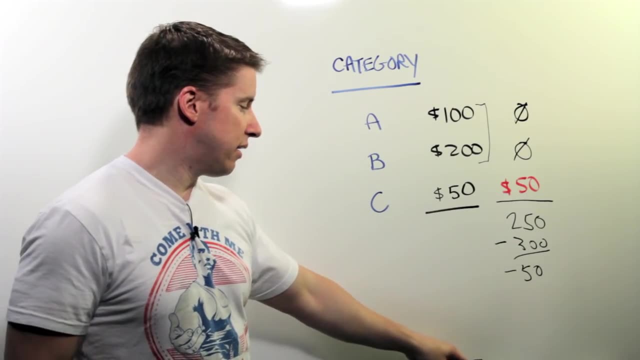 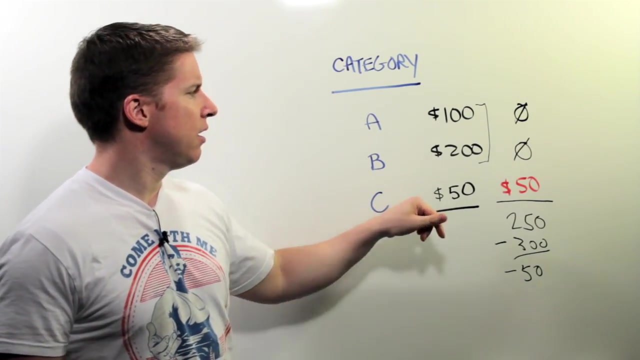 This happens when your category balance is $100 overspent, $500 overspent, when three of them combined are $1,000 overspent. This is why, in what I like to call the red arrow incident, red arrow gate, maybe, arrow gate, arrow gate sounds good. This is why we killed that red arrow: because people were 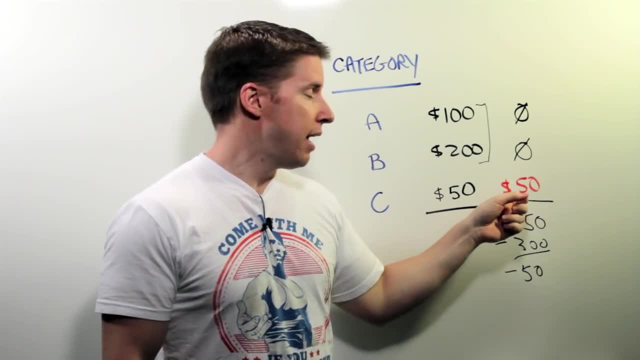 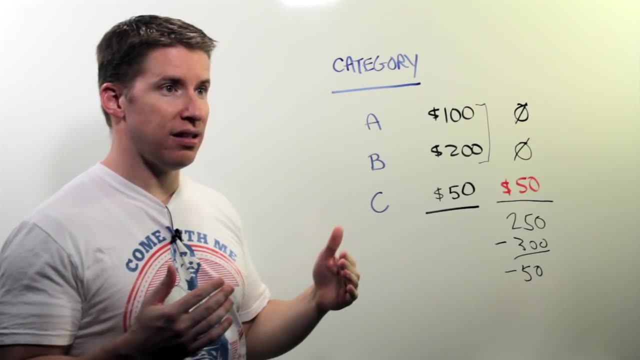 rolling the overspending forward and we were ending up with incorrect category balances. As soon as you have a penny overspent, we can't say you can go ahead and spend this money Now. of course everyone sits with a lot of 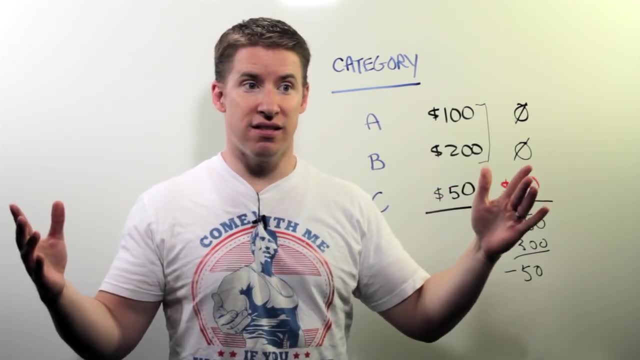 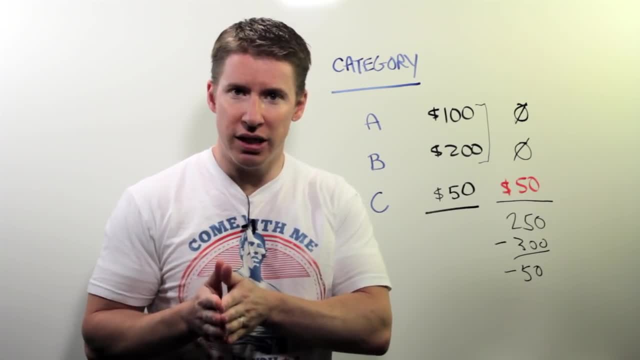 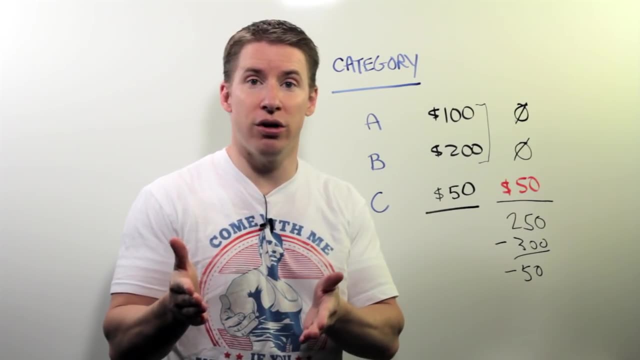 You're like Jesse, why worry about that? But I don't worry about you because you're rocking and rolling. You've been doing YNAM for a while. I worry about the person that just started and is right on the line. has $200 in their checking account at any given. 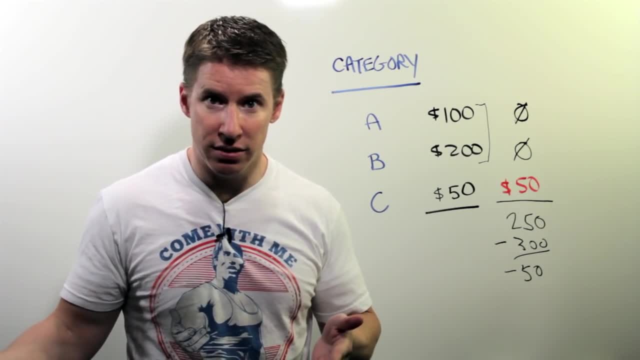 moment And we don't want to send that person off the rails. That's where we focus. So eventually we're going to have to pay them back. you guys that are experts, you're just like i do the budget, because it helps me line up my money. 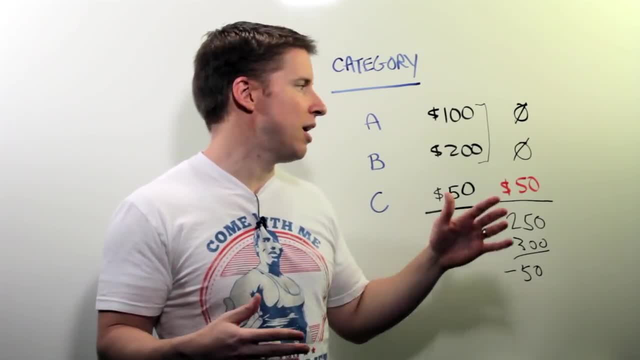 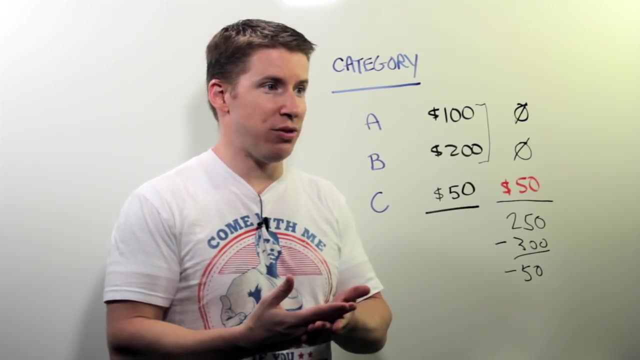 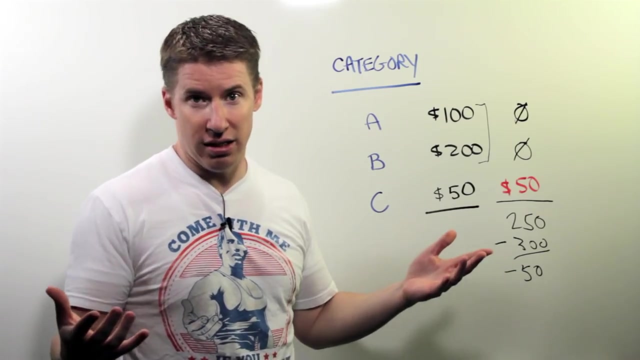 with my priorities, i feel content, my relationships may be improved. blah, blah, blah. i'm sitting on thousands and thousands and thousands of dollars in my checking account. that's not unrealistic. average wine, ever after nine months, instead of having 300 bucks in their checking account, has, on average, 3300. so it's real. everyone just sits on a lot of money eventually, and i love the fact. 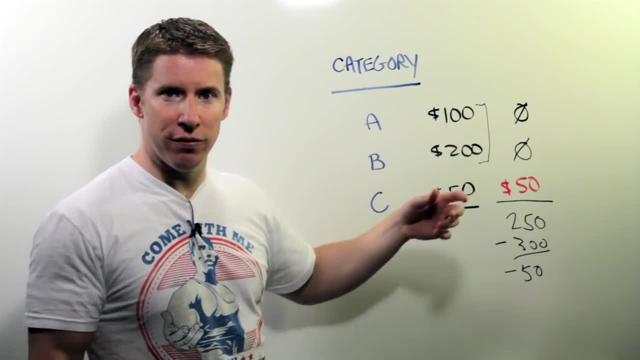 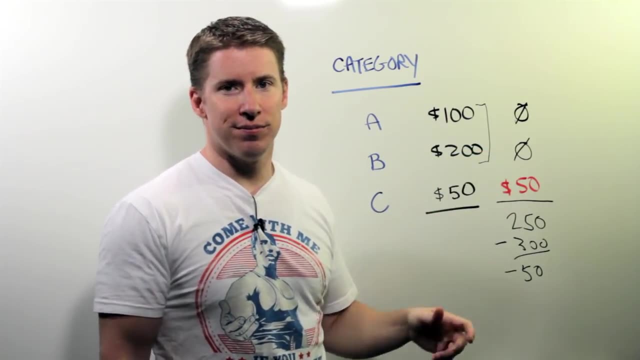 that we can be a small part of that, but this is still a problem for folks that are new and you're telling them: go ahead and spend 100 and 200, but they can't really. they really only could spend 250. that's an issue. so right now to address that, and since the beginning of YNAB- well, almost there was. 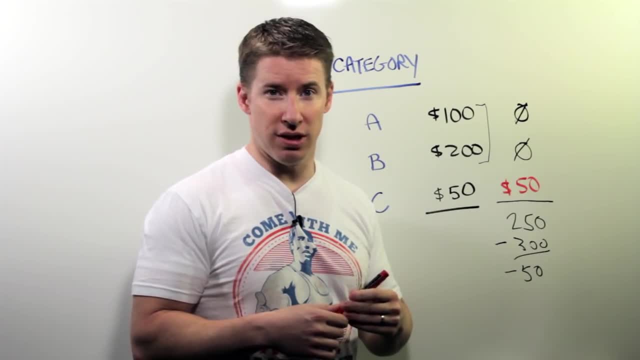 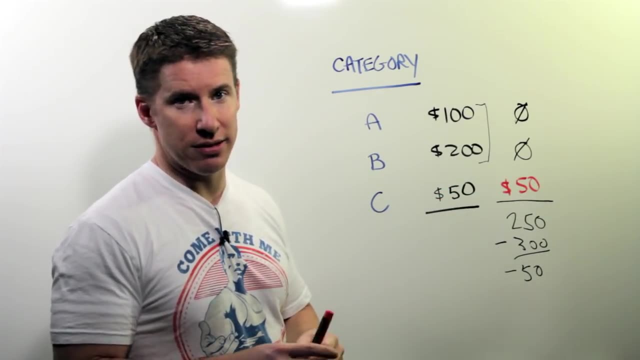 about a week when i wasn't selling it to anyone and it was just me and julia using it and i noticed this problem early on. but to make sure that you don't roll those forward and constantly having incorrect category balances, we do what with that to be budgeted up at the top right. we call it tbb. 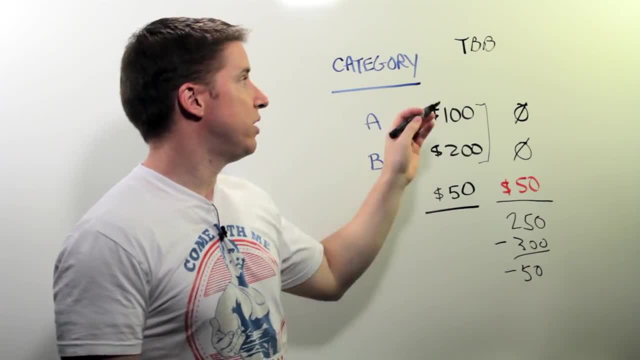 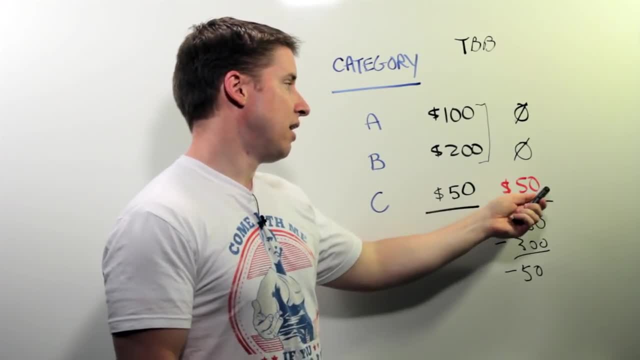 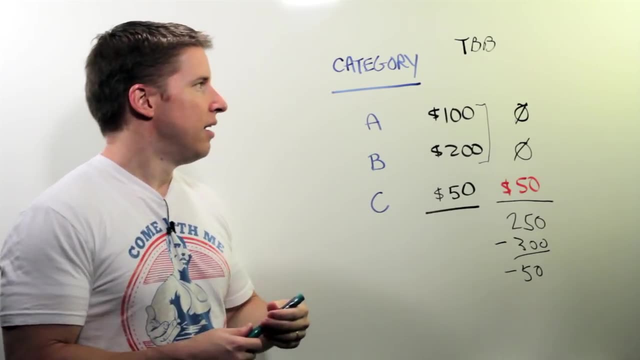 that from your next month's to be budgeted, we've been eventually say, hey, you need to pay that back so that you're, though hundred and two hundred are actually correct. the question then remains: you could have someone with incorrect category balances. if they overspend on day one of the month, they 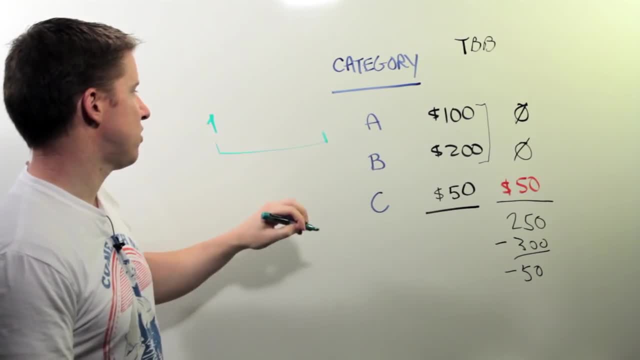 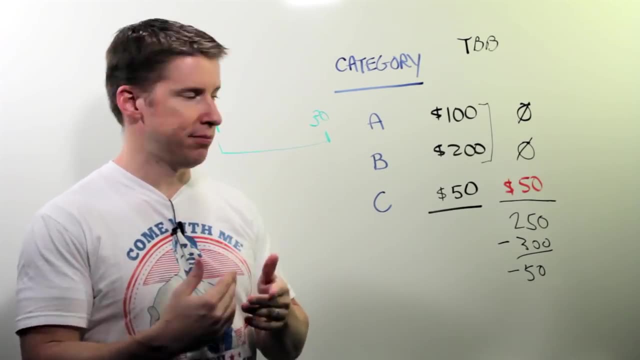 could you know, and then we don't correct it until the next month's to be budgeted. you could have a span of. did anyone notice that? I just moved here quite a bit? the card filled up, so we're back and I've emptied the card and I'm back in. 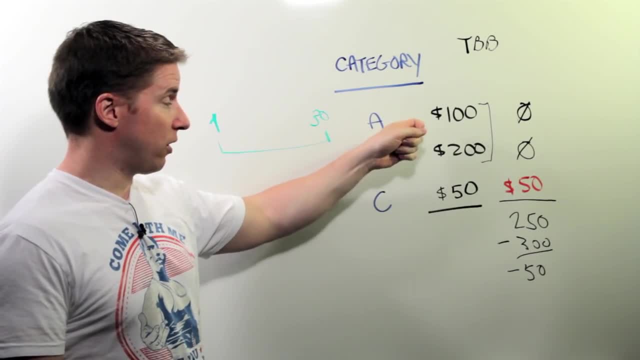 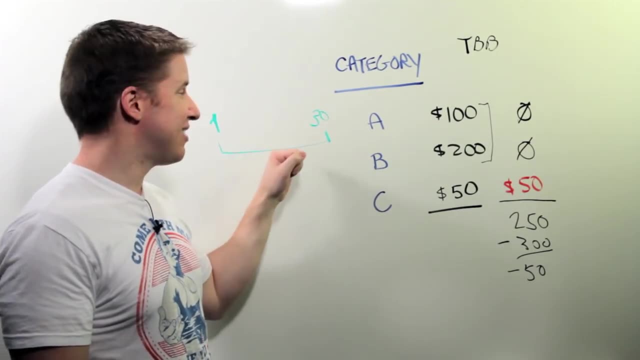 action. this is a long one, but it's important. someone could have incorrect category balances basically for as long as 30 days, or if the incorrectness happened on day 29, maybe just one day. essentially, they have incorrect category balances as long as they haven't yet been paid and put that into to be.